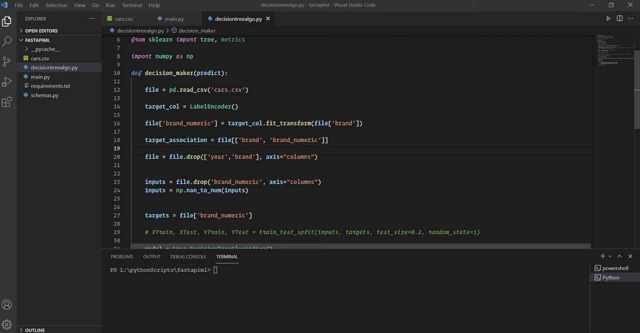 Hello everyone, Welcome back to my channel and this amazing video. I'm Aditya. In the last video we saw about how to create a decision tree algorithm and connect it with our Nuxt app. So we use FastAPI for that. So what I thought was it would be great to just compare other machine. 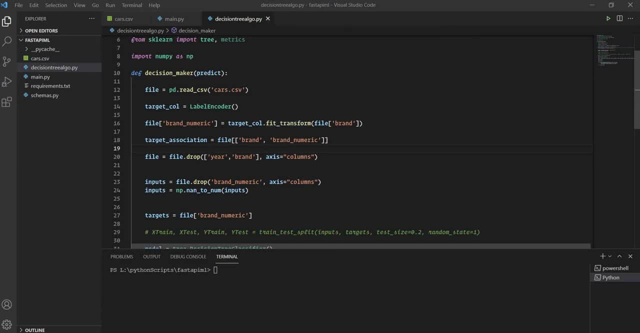 learning algorithms, So mostly the classification algorithm. So I thought maybe we can compare decision tree, random forest, KNN and neural network and also maybe knife base classifier. So I won't be dwelling in the detail of each algorithm, So I'll assume that you have the 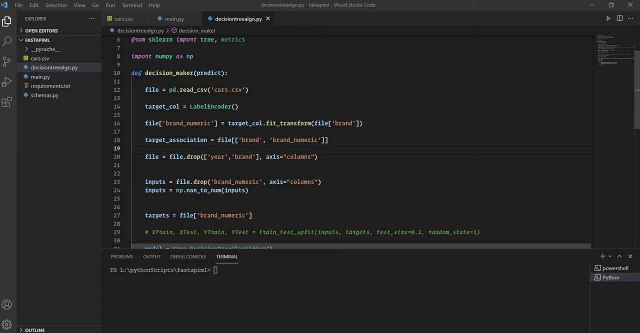 knowledge of them. I might tell you in brief what each algorithm means. So what we are going to do, we will just use this to just get to know, like which algorithm is best in this scenario, or which algorithm should be used for our scenario. So let's get started. 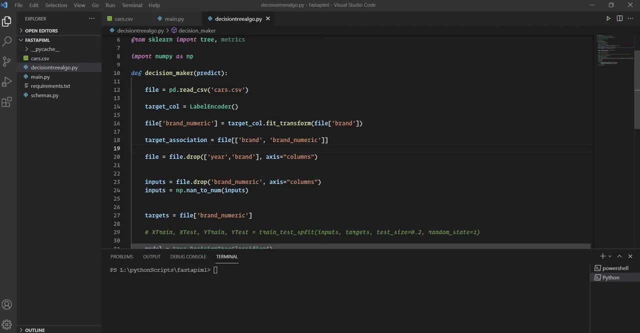 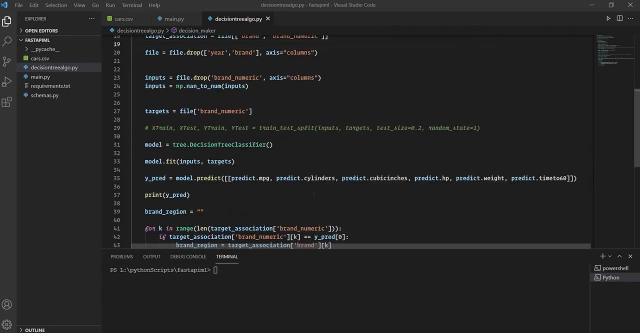 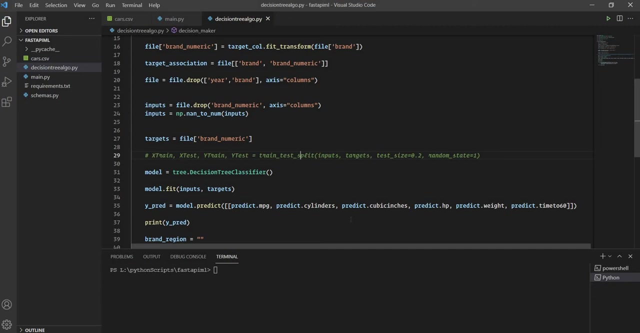 Also, there are various amazing ways to get the best algorithm, So I came across another one which was K fold cross validation. So that's another way, But here I will be using train test split method. So I'll be splitting the data into 80% training, 20% test. 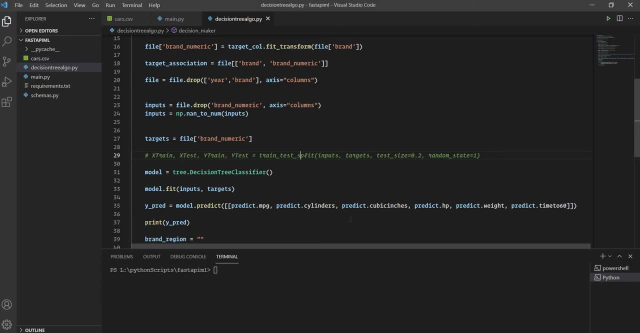 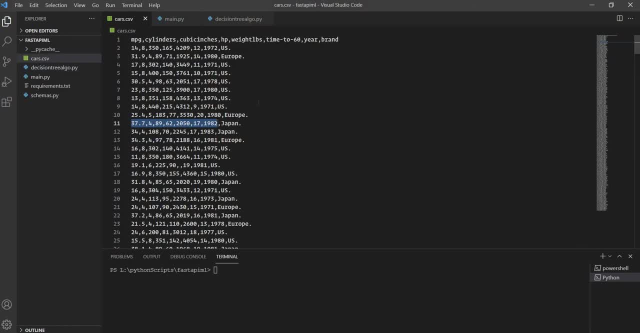 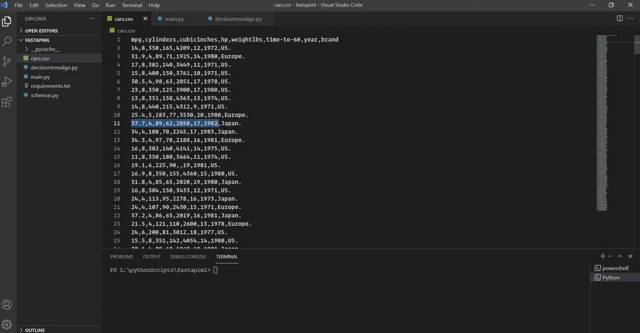 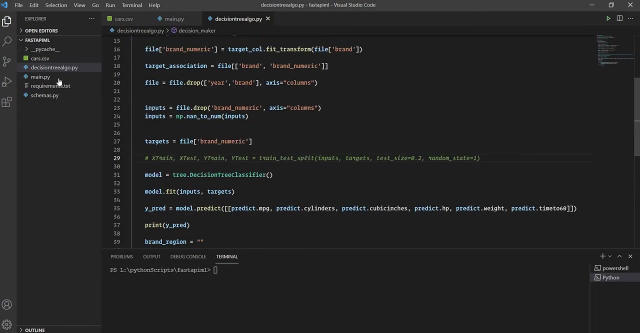 the description below. I will put it over there. So in that we are using this input parameters- except the year- to predict in which country the car should be made. So so far. so it's all working great with decision tree algorithm And let's now rewrite this function. So what we will do? 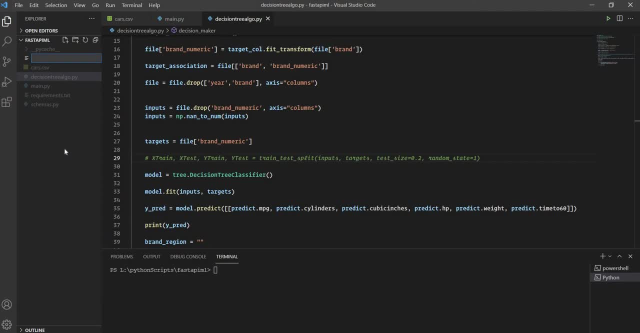 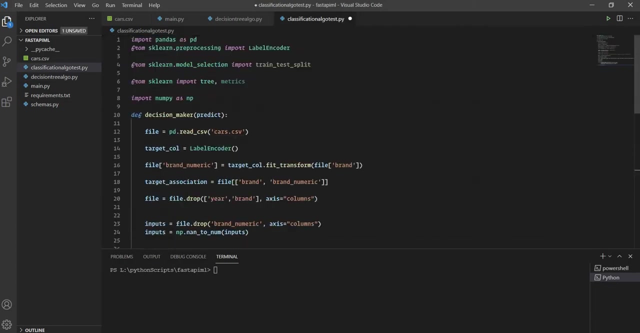 is, we'll create another new file, So we don't disturb this file. So we'll say classification. So we'll say classification: Algo dot, PY. It's a long name, So let's copy and paste it over here. Or rather, it could do a class based approach, but it's okay, I could create an algorithm class. 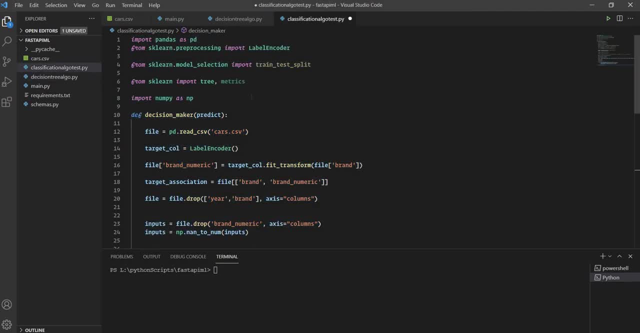 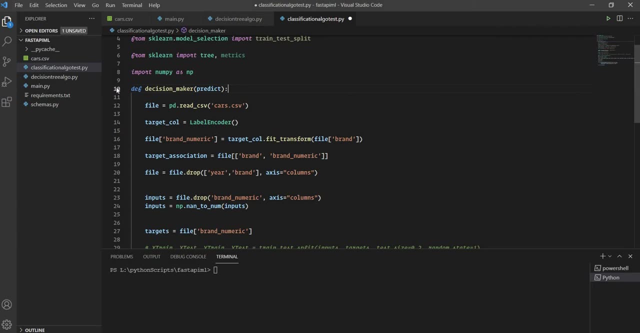 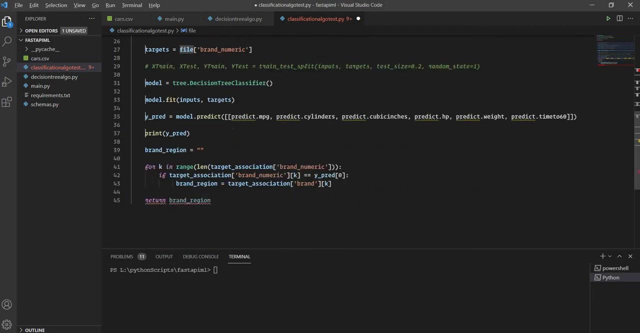 and then call those class individually over here. That's fine as well, But let's do with only simple thing. Let's keep it simple. So what we need here now is we don't need this function, of course, so let's uh do like this. so we need to always like: just do it over here, we don't need these lines. 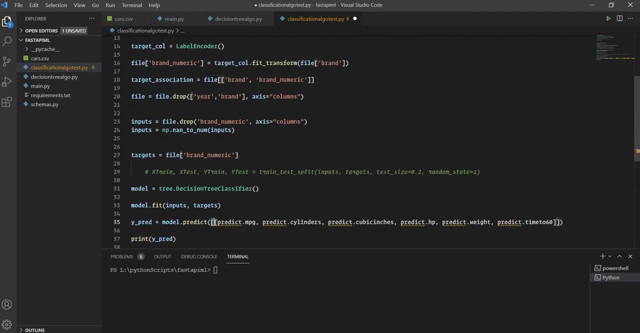 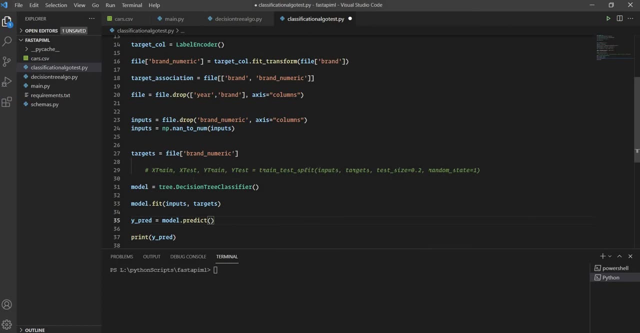 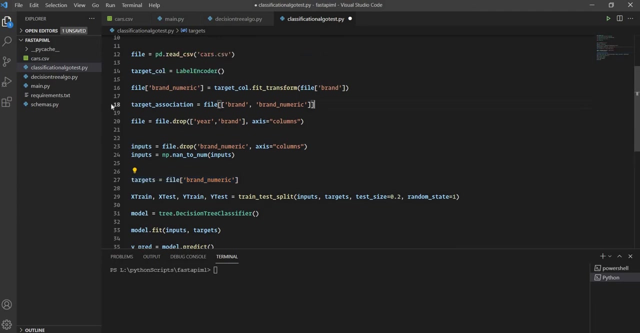 because we are not doing anything over here. uh, we will just remove this for now. so we don't need this and we have the cast or csv. that's fine, and we will need this line as well. uh, targets brand numerical: keep this and yeah, this target association is no more required. so let me tell. 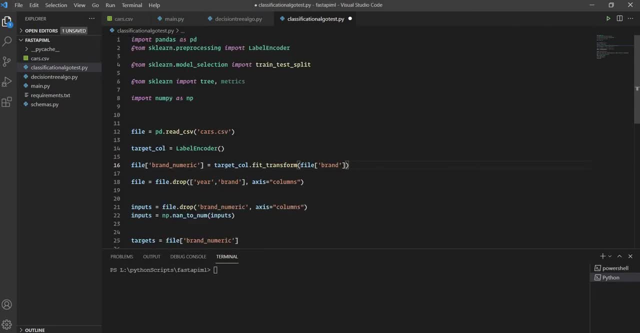 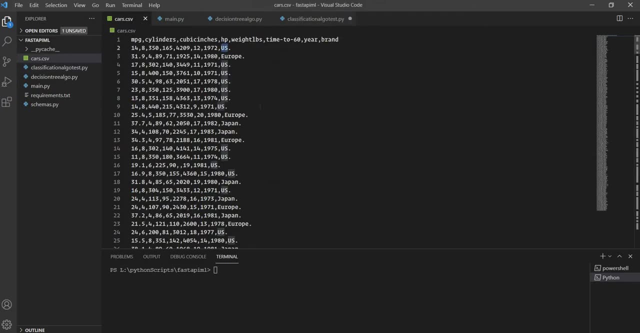 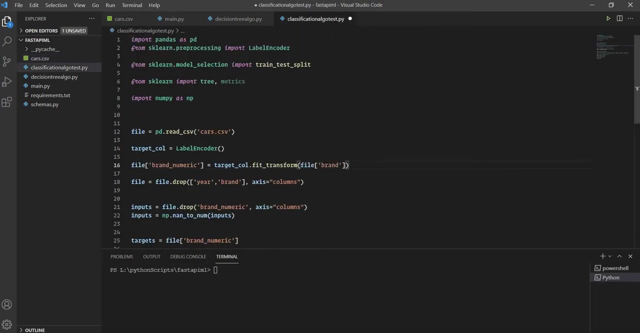 you in quickly what we are doing here. so we are importing pandas, we are importing the file using pandas, so it's a csv file. then we are encoding the label because system understands only the numeric language, numeric values. so this us, europe and japan. as there are three classes, they will get a numeric values. with this label encoder we are dropping. 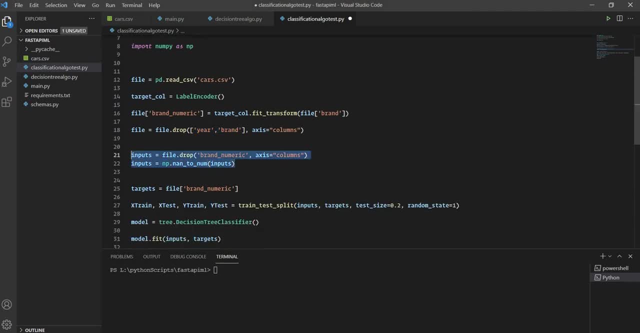 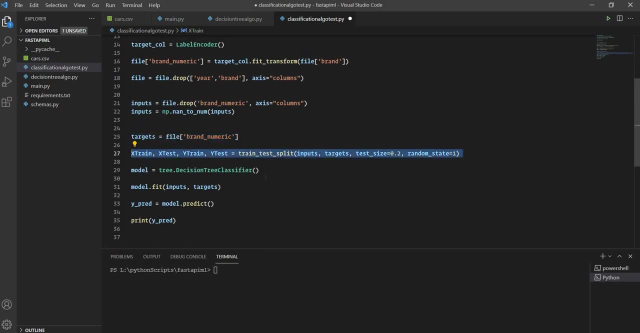 the column of year and brand. then we are refining our input. we are then setting our targets and then just dividing the data into training and testing for each input- train input test output. train output test- and then we are just using our uh models. we are first initiating the instance of 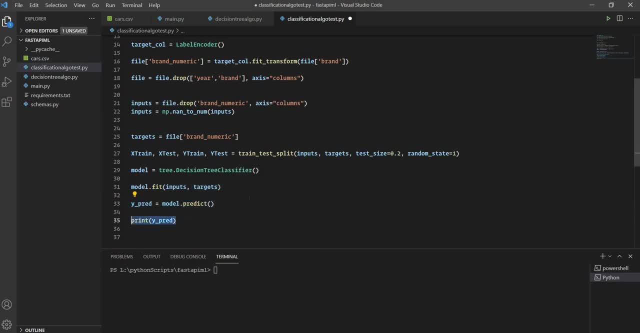 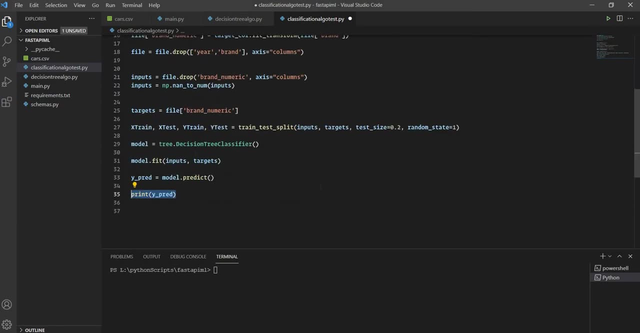 the model, then training it over here and then just predicting in and that result, printing the. so that's pretty simple. so the tree we have decision tree classifier. so let's now let's change this to decision tree, decision tree model and let's do over here as well. decision tree model. 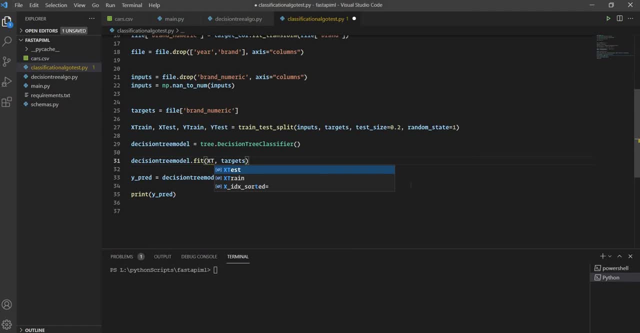 and here, instead of input now, what i'm going to do: x train, so i'll be sorry, not trade test for x train and y train. okay, and here i'll be predicting the result using our test data, and here i will say by predict, i'll say y, decision tree. okay, now let's print the. 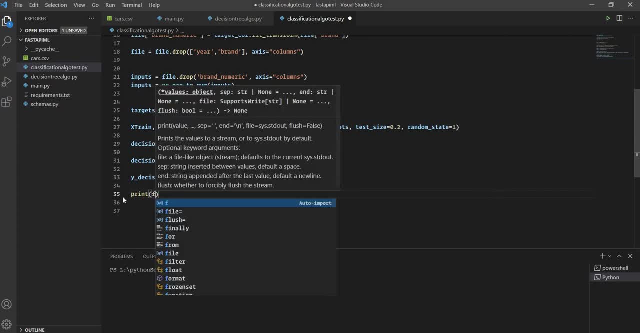 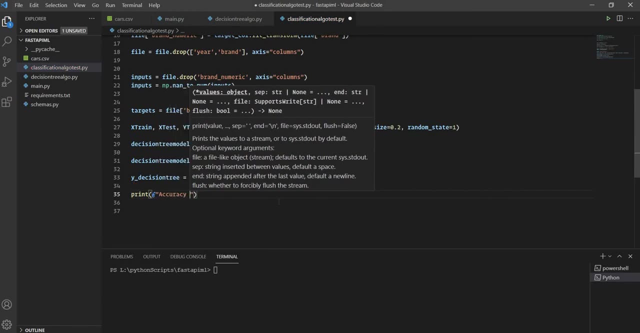 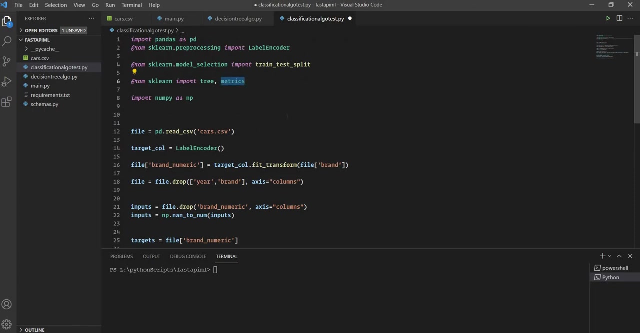 core object. so i'll say pin, and then i could sorry, and then all i need to do is accuracy of decision tree. algorithm is: let me spell it over here: so it is and what will be the accuracy. it will be nothing, but so we could use the metrics from sklearn. it's an amazing library, so scikit it's. 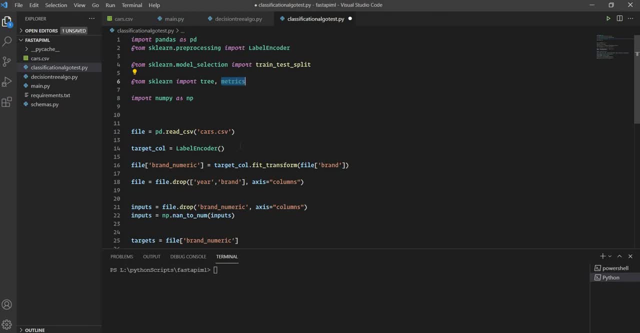 an amazing library, scikit-learn, in python to use all the possible machine learning, more algorithms we could so, and it's make it pretty simple like you can: the testing, the scoring, the usage, the training. it makes it pretty, pretty simple, so let's use that. so we will use the metrics from: 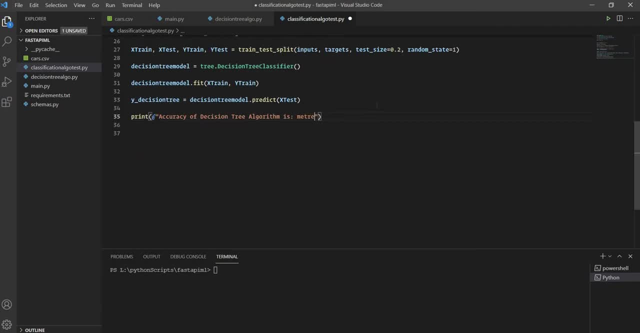 this sklearn and we'll say metrics. sorry, it should be like this. there's a metrics dot accuracy score and what we want to score against. so we want to score against our y test and our actual prediction, which is y, decision, prediction, decision tree, this one, this is our. 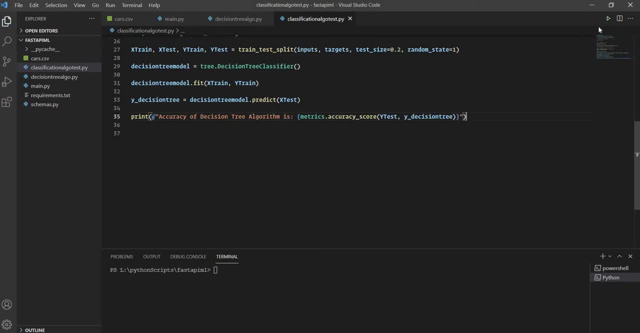 actual prediction. this is our test prediction. now we will see what do we get from this. so if i run this, we are getting the accuracy of 0.77. so let's do it into like: let's multiply this into 100 so we get out of 100. so if we'll get it in, 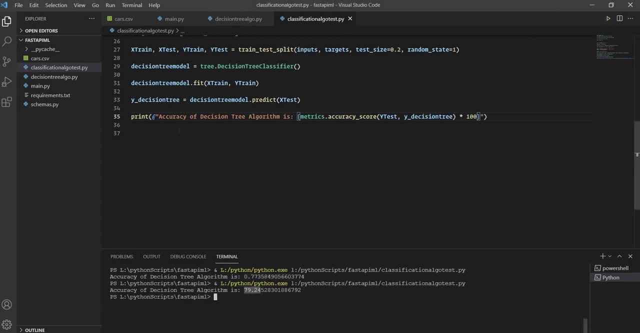 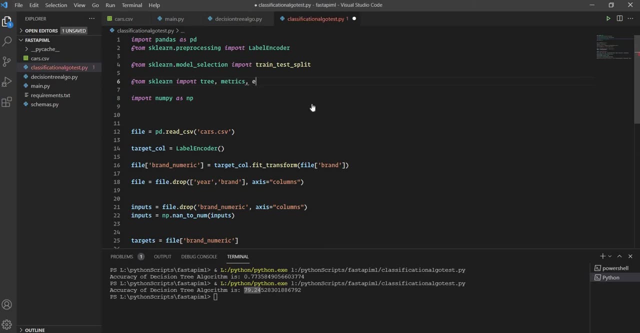 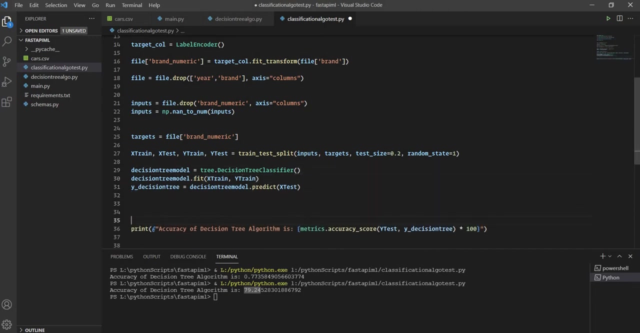 percentage, simply so we are getting 79 of accuracy. now let's do the same. now let's strike for random forest. so from sklearn we will import and symbol and here. so let's club this together so we know that this is a decision tree. now let's do it for random forest. 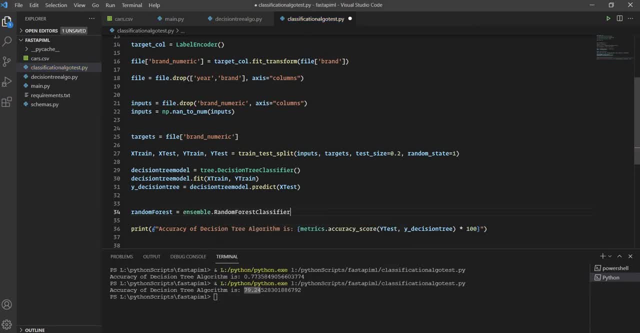 equal to- uh. this will be ensemble dot random forest classifier. we are dealing with the classification algorithms so we'll keep it simple and default states for all. so random forest dot and then x train and y train. then we will have y- random forest equal to random forest dot predict and that would be x test. 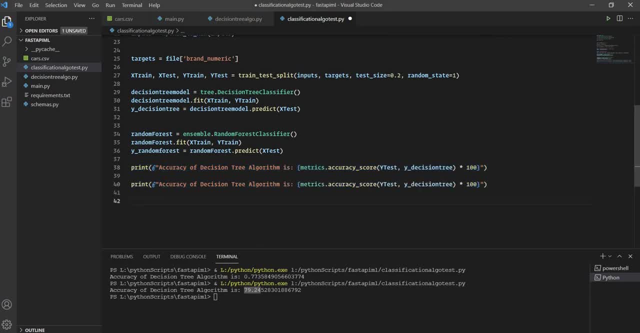 and then we'll just copy this line and print it over here and here, instead of accuracy score of y decision tree, we will say y- random forest, and here, instead of random decision tree algorithm, we will say random forest algorithm. okay, so let's see what we get. let's run this quickly and it will take a bit of a time, and 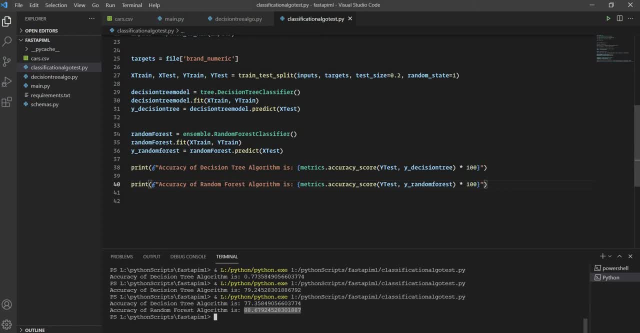 you'll see like the random forest has way higher accuracy than decision tree algorithm. of course, once you have more amount of data, these values will differ, and in train and split these values definitely differ. so if i do it again, you'll see the values will differ. so 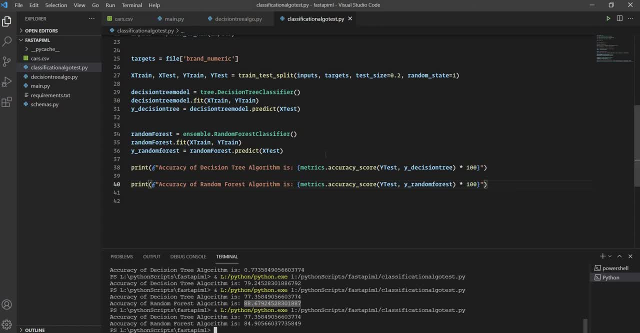 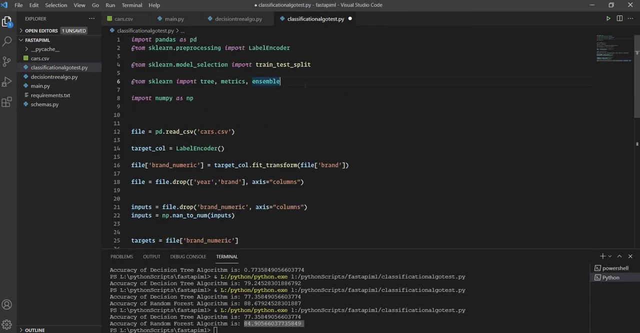 it depends upon, like, because this splitting is random, so it's kind of like: uh, the accuracy will be different, differ here and there, but the main point would be: here is random forest is doing way better than decision tree. now let's see another algorithm and let's do it quickly. so we'll do neural networks. 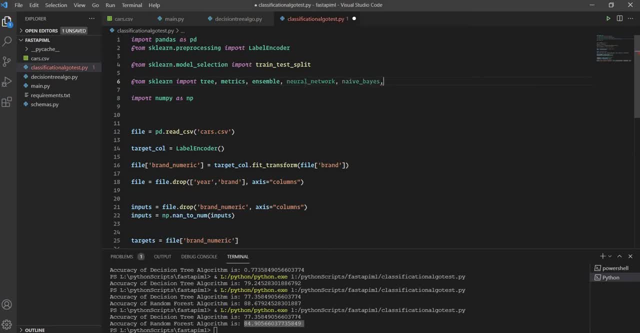 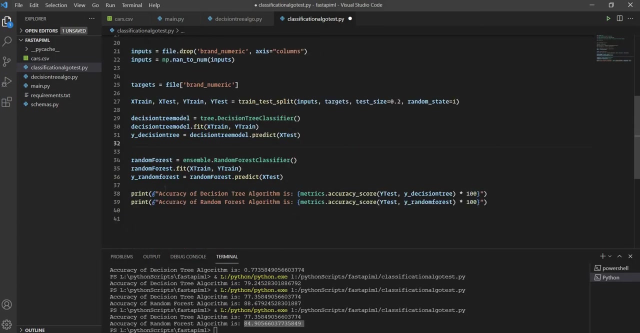 then we will need knife base and let's try knn as well, so nearest near neighbors. so we are including from sklearn, we are using neural network, we are taking knife base and we are taking neighbors. these neighbors will be for k: nearest neighbors, knn algorithm. so let's go over here and let's copy these lines and we will just need to modify them. 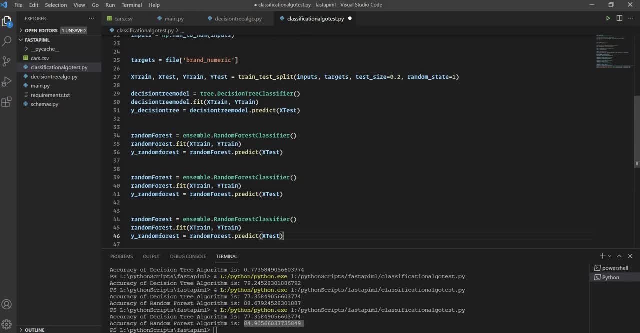 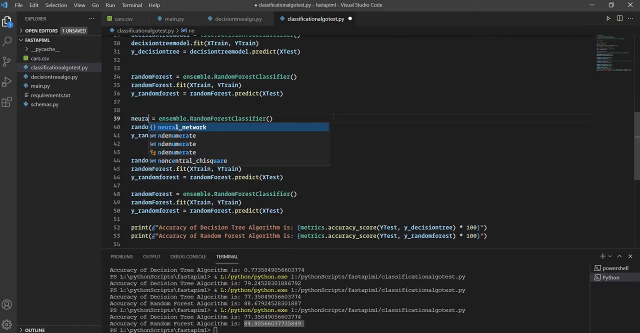 so one set for a nearest neighbor, one set for knife base and one set for neural network. so we have random forest here, so we will change this to neural network. uh, it will be problematic. so here we'll say neural network and here we want. so i'll just remove this. 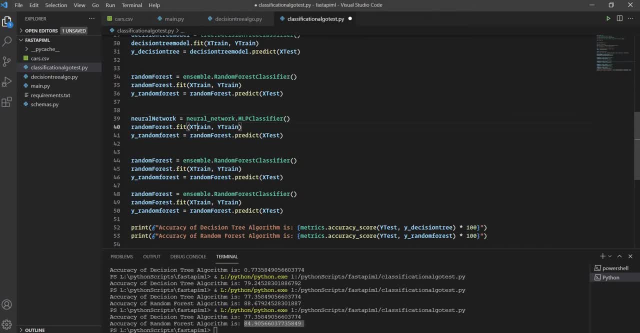 we want mlp classifier. so once we have this, we just need to copy this over here here. so this should be over here. let's do y and then for neural network and then predict with the neural network. after that let's try for night base, so knife base. 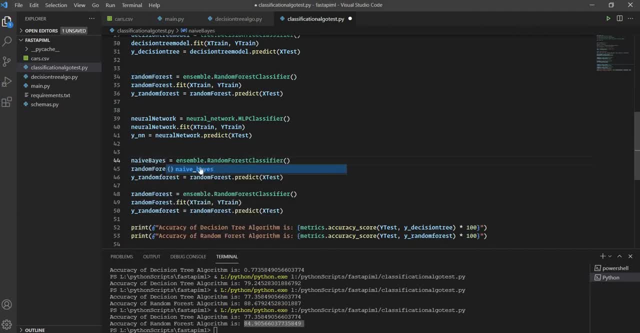 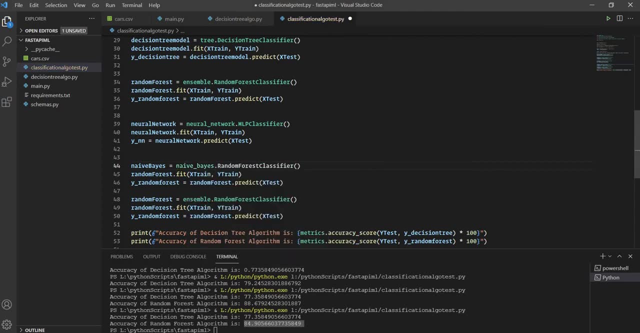 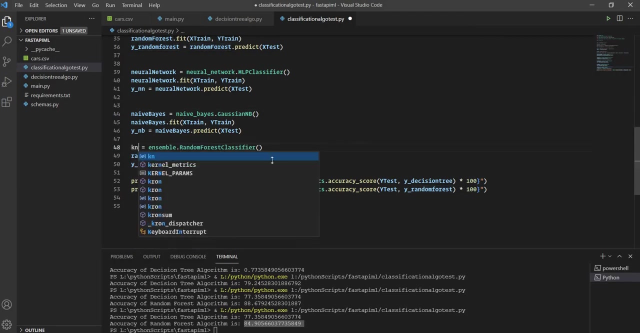 and here we will use these knife base, so it's a knife base, and we will be using the gaussian knife base classified, so gaussian knife base classified, and then we will just paste it over here here and let's do this nb last. we need it for nearest neighbors, so let's do knn k- nearest neighbor. 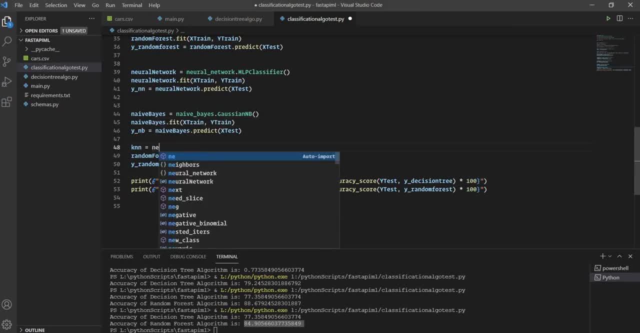 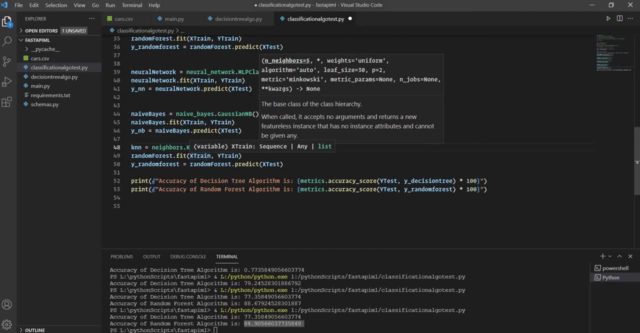 and here we will need to use neighbors dot k, nearest classifiers. i can give the value of nearest neighbors, so i'll put it by default five. so like i guess it's by default five, i guess. but let's do not give any value and let's see how knn algorithm gives. 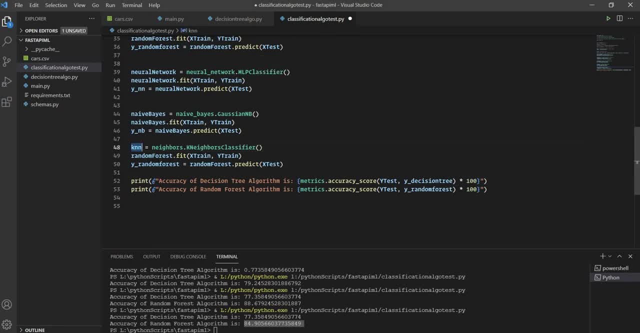 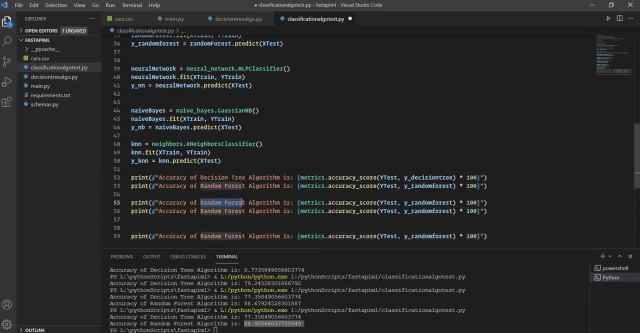 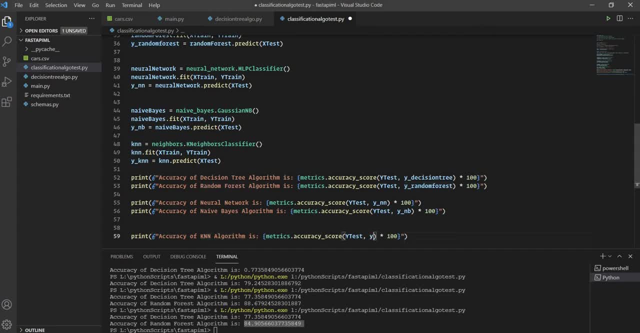 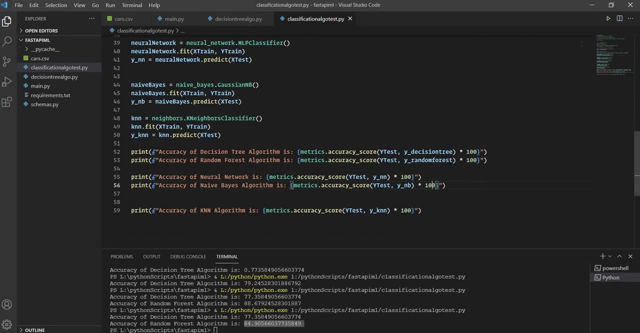 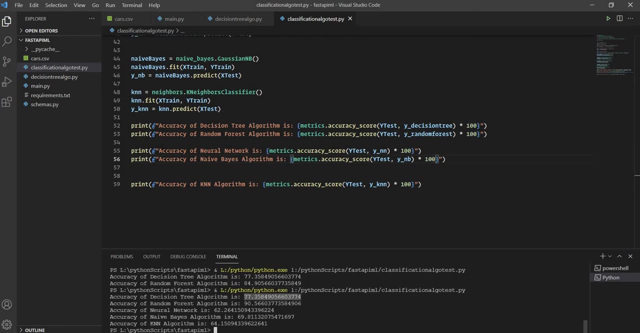 result of knn, this would be y knn. now, what do you think? which algorithm would have the highest accuracy? so let's see, so let's run this and if you see, decision tree has 77. almost random forest has 90. neural network has 62 percent. knife base has 69. 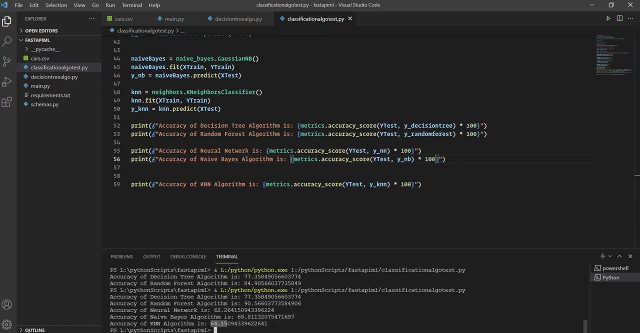 almost 70 percent, i would say, and knn has 64 percent. so if you see, random forest is doing way better over here, so that's it's. uh, like it won't be fair if i don't say what exactly random fire algorithm is, so you can. 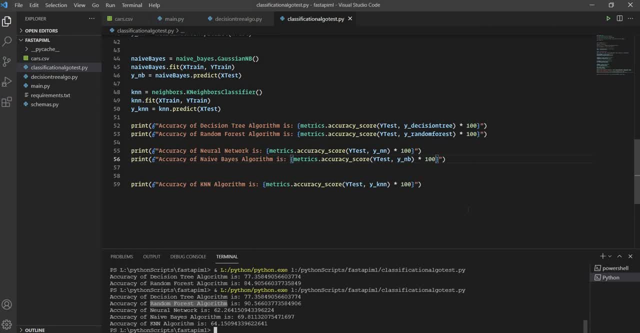 consider it's nothing but a collection of lots of decision trees and when it comes to classification, it uses or it makes the prediction based on those classes which gets the maximum prediction from each decision tree. so suppose there are five decision trees in any random forest and each 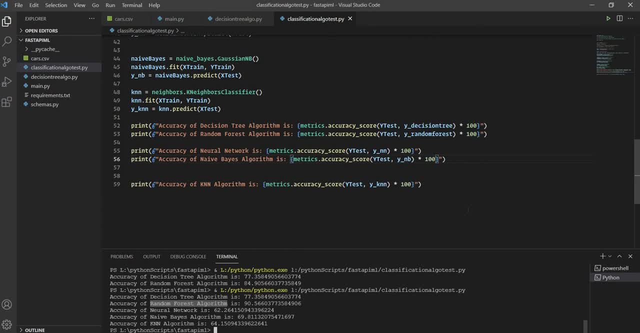 then there are two classes. let's say yes or no. if three are saying yes, two are saying no, then it gives yes as a higher vote. it's in very, very simple words. in mathematically speaking it's a bit complicated, but in simple words it just chooses the best possible like like the one which 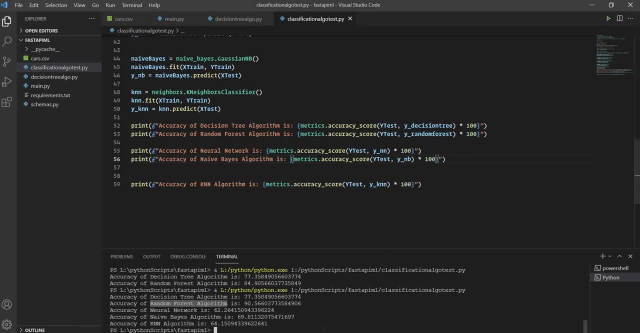 gets which one class which gets the highest score, it comes as a uh winner. it's as good as saying: when you're going somewhere for a travel, you ask several, several of your friends like where to go and the place which gets most of the votes from your friends, you choose that for your travel. 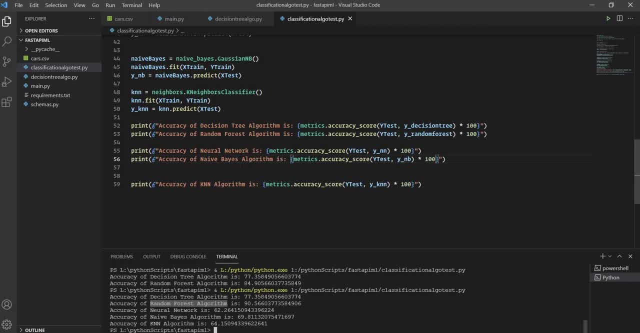 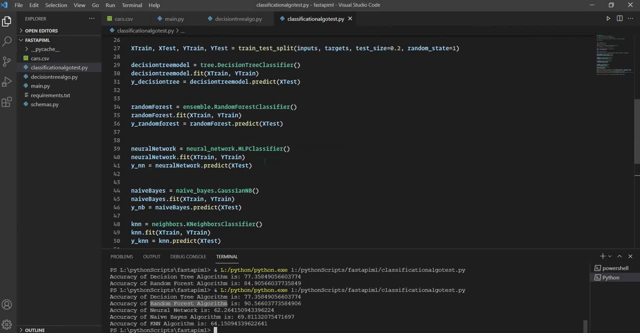 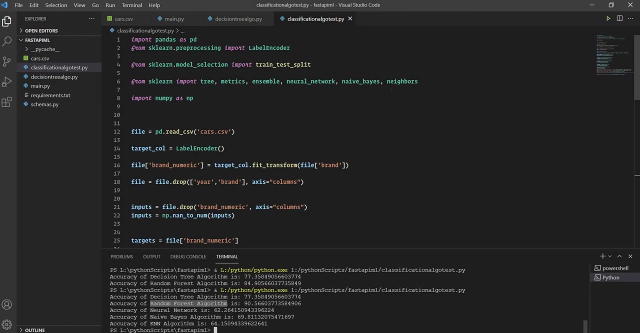 destination. it's same with random forest, so it's the same thing, uh. so i guess that's pretty much it for this video, so i'm not sure if i have missed anything. so, uh, metrics ansible. okay, we haven't tried, uh, the svm algorithms. let's try that as well. so let's do, uh, i guess it's svm. 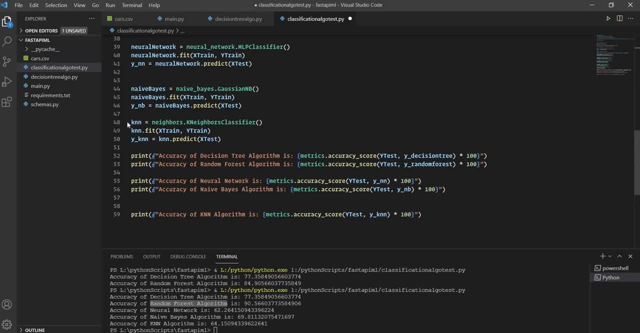 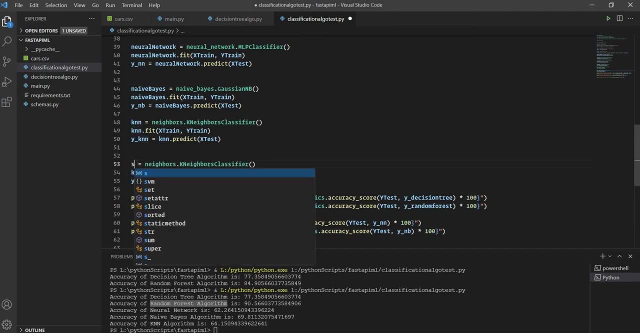 from sklan. so before we conclude our video, let's try for svm as well. so here i'll just copy this. i'll say svm. i'll go: uh, naming convention is going here and there, but that's okay. so, let's sorry, i did something wrong. no, so here now let's do so from svm. we need to get dot svc. 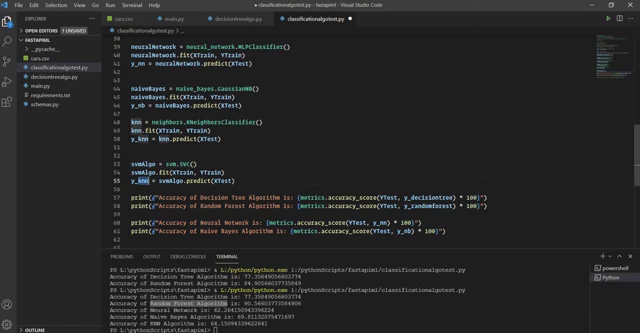 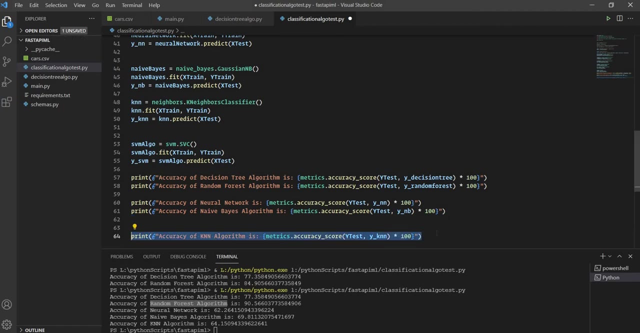 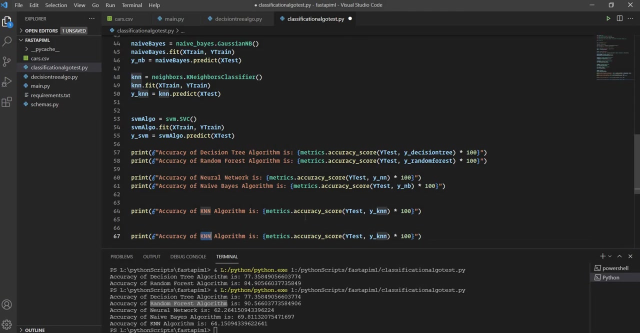 so we will need to also change the heat over here. so let's say: why svm, sorry, svm. actually, you know it's okay, we will add some data and then we can do a little bit of my own and let's do the prediction for that as well, of the accuracy score, actually. so 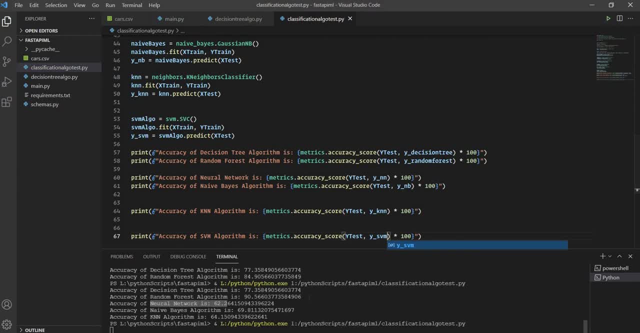 let's go over here and svm. then we have the accuracy of y svm, and now let's see how much accuracy this algorithm gives to us: 4.0mfpw.2.4.4.3,5.0.5.5.2.0,4.5.5.6.4,4.5.5.6.4.5.4. 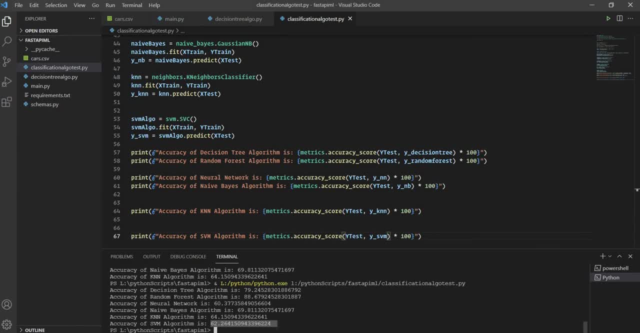 SVM here is giving around 62%. so it's but obvious, like, mostly like when it comes to classification, it's generally random. forest is mostly used and yes, I wasn't surprised with the SVM result because I knew that it will give you, it will give the less accuracy. but I'm a bit surprised, like neural. 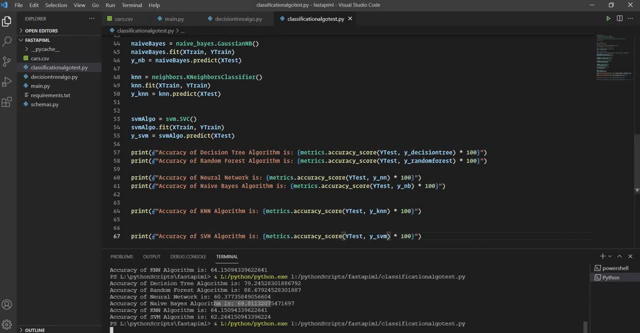 network is giving more lesser accuracy than SVM. let's try again one more time. so if I run again and neural network is 58 while SVM is 62, yeah, this is a bit surprising for me. so let me know in the comment section why do you think that this is like which one was surprising for you? 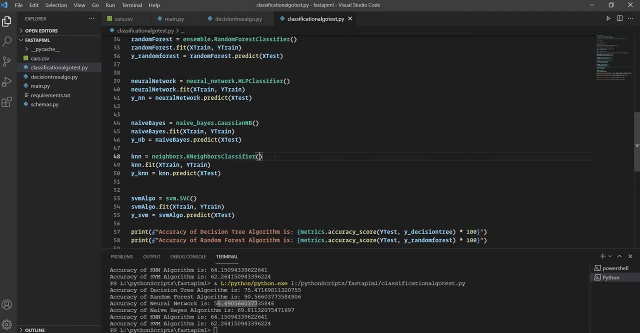 also, let's try with the KNN. let's try to change the nearest neighbors. so let's say n- I guess it's neighbors- and then let's try from two and let's see KNN value for two neighbors. so 71%. let's run again 71%. let's change the neighbors to four and let's see what we get. so 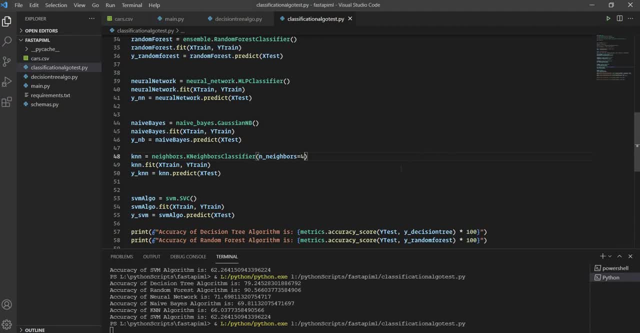 okay. so as we are going like, as we are increasing the value of K, the accuracy is going down and down. so let's see so 71, okay. so I guess the best value for here is two to three. so in that range. and yeah, I guess that's pretty much it for this video. hope you enjoyed this video, if you feel that.